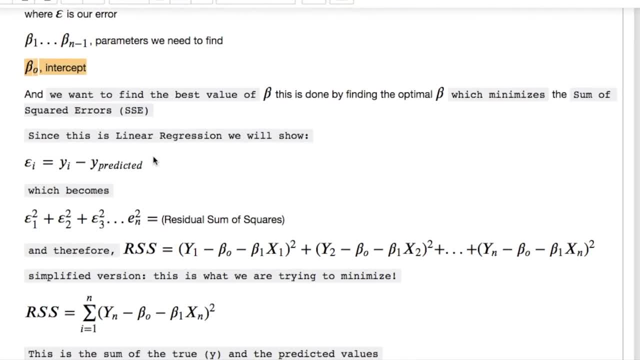 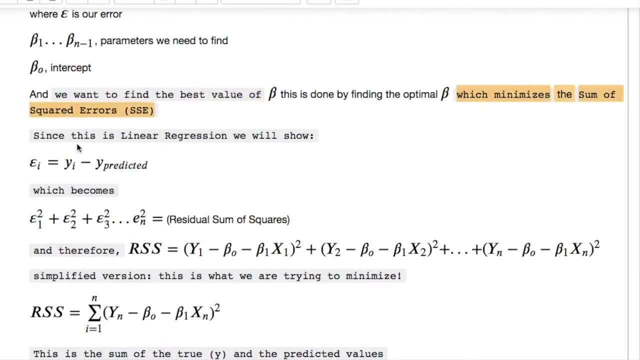 beta and our intercept of beta naught And we want to find the best value of our beta Which is going to minimize our sum of squares error. Since this is linear regression, We will be able to say that our error equals this right here. You need to consider that. 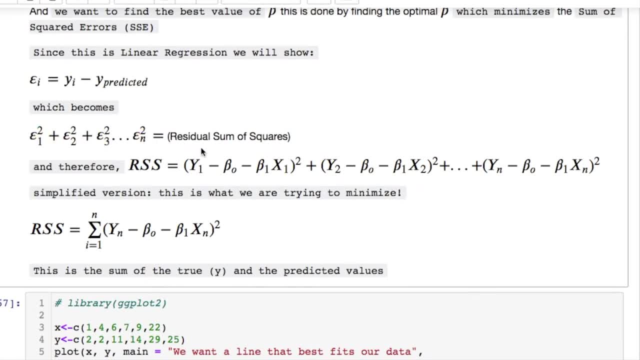 your errors are going to be added together So we can achieve our residual sum of squares And therefore- and you need to realize this is what's going on- The simplified version is this, of course, Where we're summing everything together: The sum of the true y and the predicted values. Now let's look. 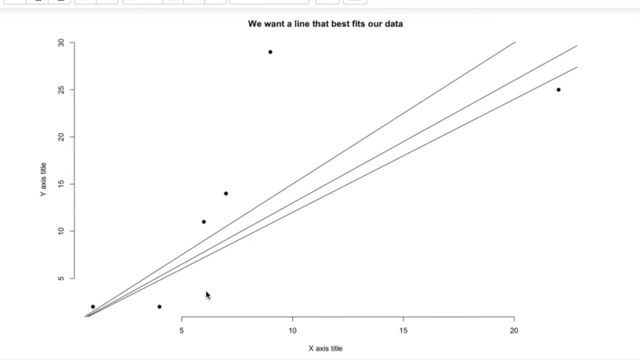 at this one. So we're trying to basically acquire the best fit line for our given data. So we're trying to basically move this line around to minimize the error that we have, Which would be the distance between this line and this point. Now, the next thing i want to show you is i ran a. 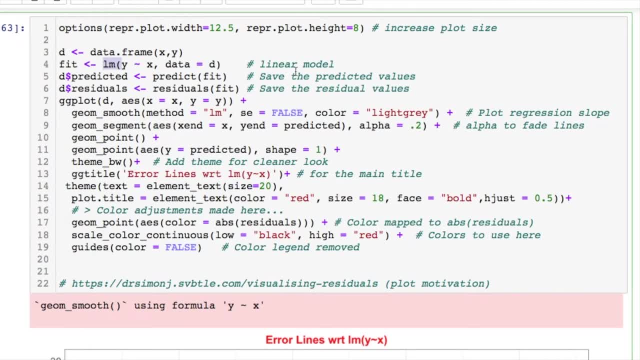 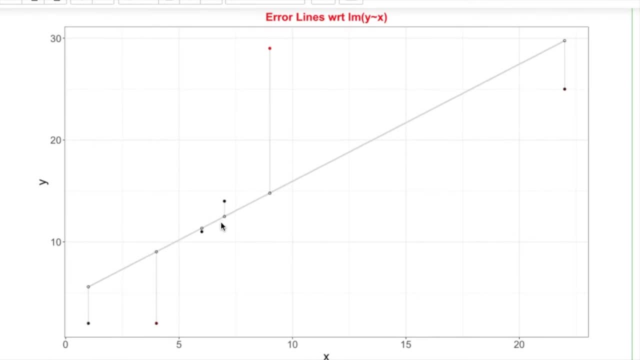 linear model with those made up data i had before, Which you'll notice right here. If you want to pause the video and see how i set that up, feel free to do it. But this notice something. I set this line, I showed the error lines for this And this is approximately the best line. 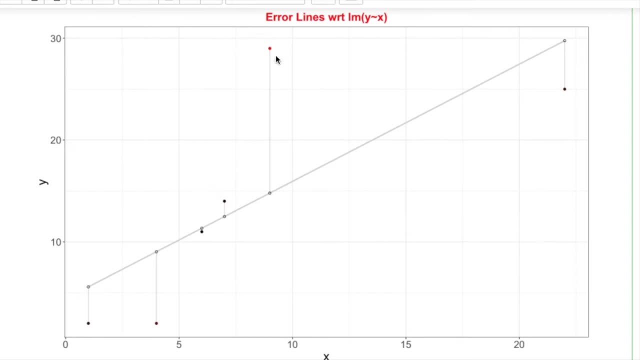 For the given data that we have. And if you see this red dot, This dot is one of our outliers With linear regression. this is kind of a problem And it will shift your line, So you have to be aware of that. Also, i want you to notice something here: Look at where this line is. It's not at the origin. 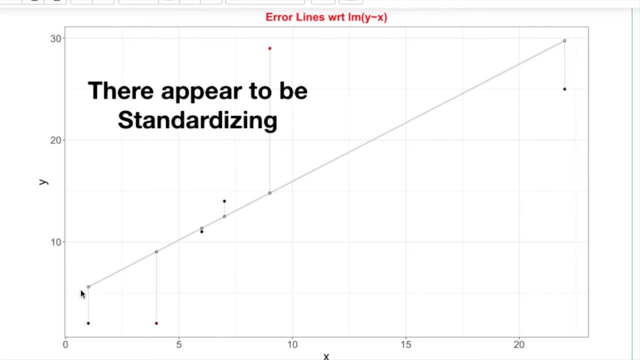 anymore. It's shifted up, So you've had some scaling or standardizing and centering of your data. That's something you should always look into And consider, for instance, if your data are on varying scales. Be aware of that And always keep that in mind. 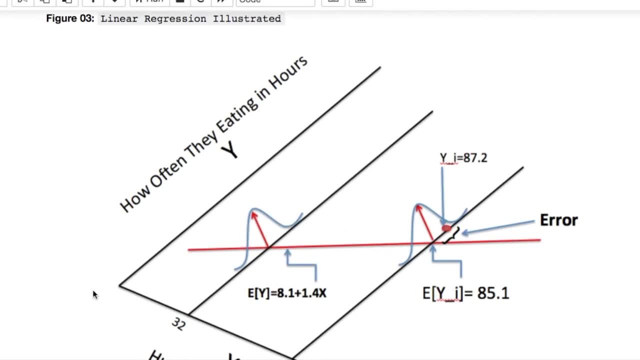 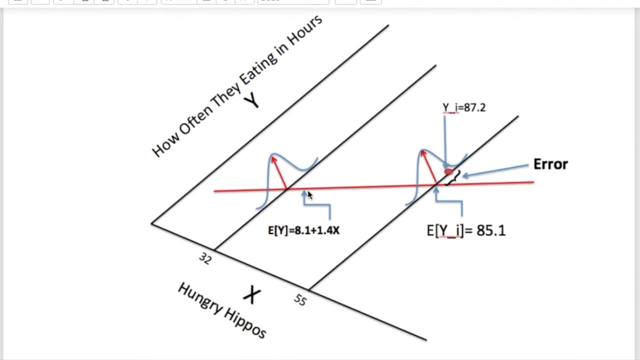 Keep that in the back of your mind. Now, this plot that we have right here is our linear model. I'm going to explain what's going on here. Zoom out just a little bit for us So we can see what's going on. Assume that this red line is our best fit line And this red dot right here is our actual. 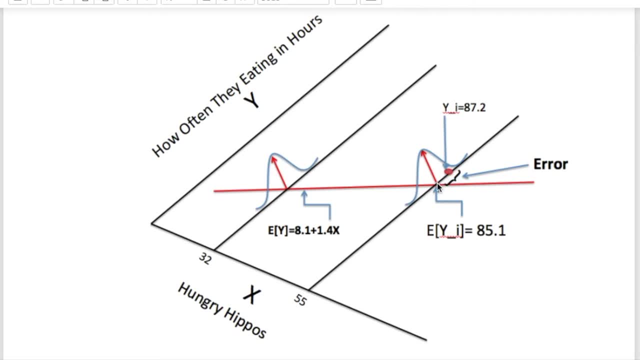 point And the distance from this point to this line is our error And we're saying that our estimated value, Which should have lie on this line, should have been 85.1.. Whereas the observed value that we have is 87.3.. 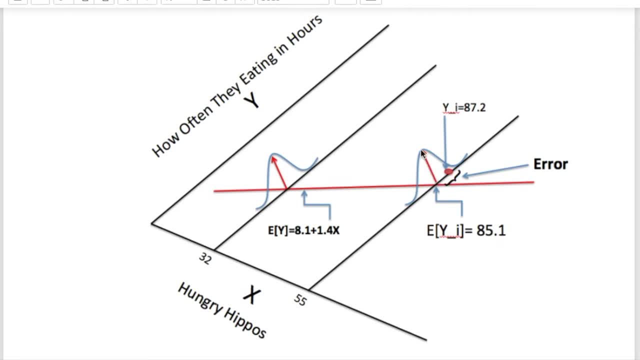 Okay, and you'll see that this right here, our expected value should have been the mean, Which would have been the peak of this right here. That's just what's going on And here's our line equation. This is telling us that these were the specific parameters that best fit our line with. 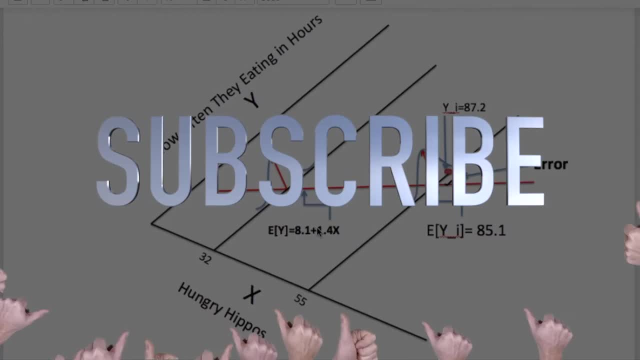 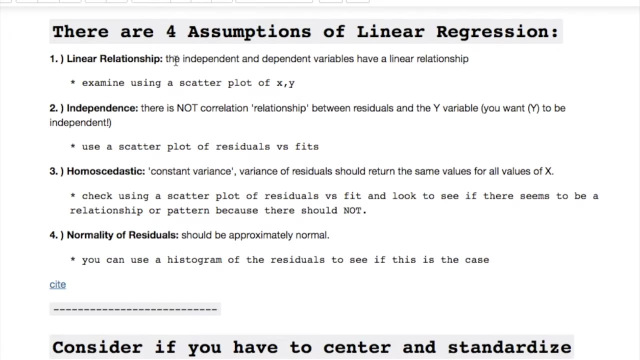 this intercept. That's all that's going on with this. to give you an idea, There's four basic assumptions for linear regression that you need to be aware of if you're not familiar. A linear relationship: So you're checking that the independent and the dependent variables have a. 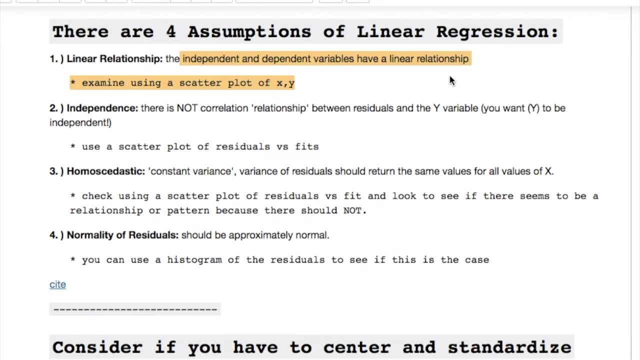 linear relationship. You could check this out by examining a scatter plot of x and y. You need to also look for independence. okay, You need to check that there's not correlation or some form of relationship between the residuals and the variable y. You may want y to be independent. okay, Use a. 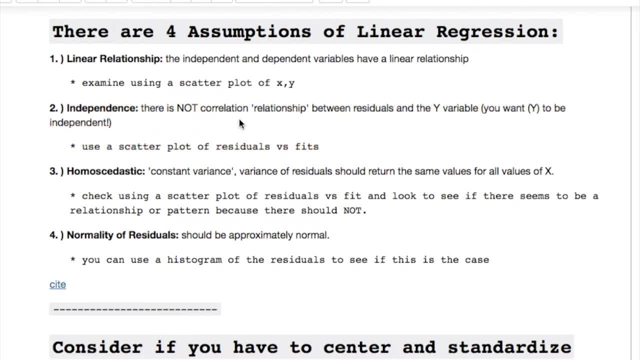 scatter plot of the residuals versus your fits to establish this. The next thing that you need to look for is constant variance. This in practice can be an issue but or unrealistic. But consider the residuals should return the same value for all values of x. To plot this and check what's going on. 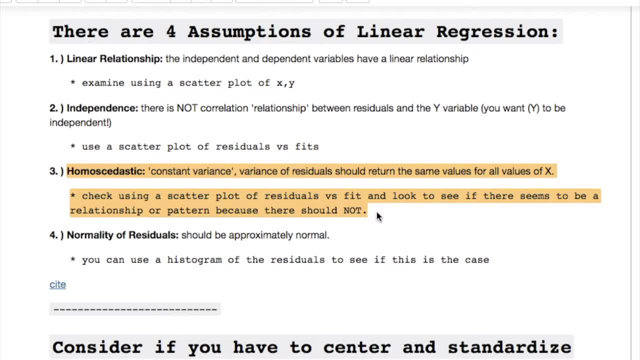 use a scatter plot of the residuals versus the fit and look to see if there seems to be a relationship or a pattern. Then you need to establish an assumption of normality. The distribution should be approximately normal. Take the residuals and plot with a histogram and see if it looks like. 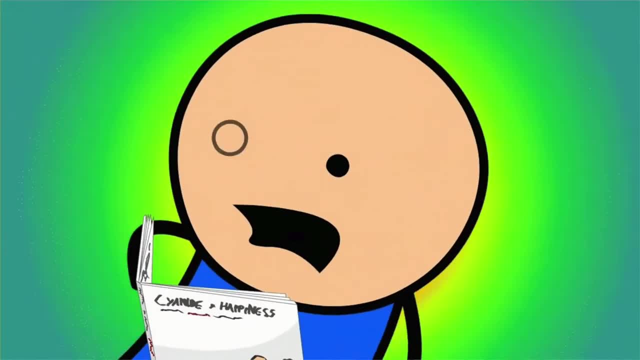 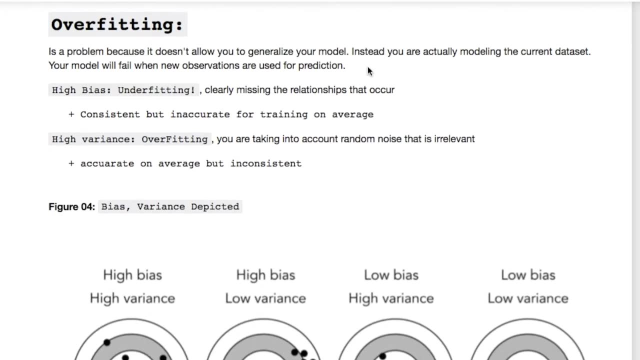 a somewhat normal distribution. This first get into overfitting, since that's what's going on with linear regression, And this gets a handle of what's going on with the distribution. So let's get into overfitting. Overfitting is a problem. It doesn't generalize your model, It's only giving you 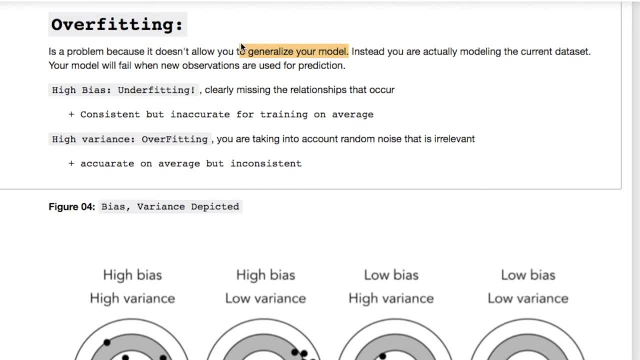 something that may be conducive for your training data. Your model is going to fail for new observations that are used for a prediction. So let's look into this. High bias causes underfitting, which will mean you have low variance And you're clearly missing your relationships within your data. 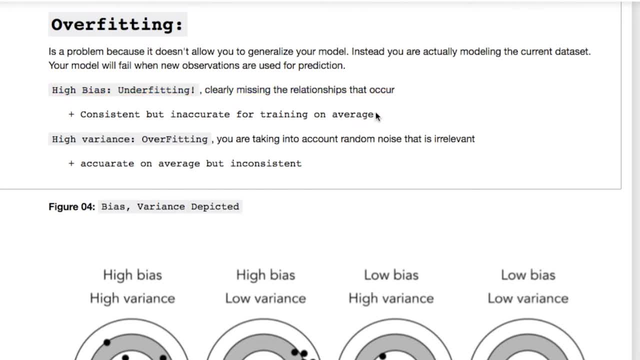 which means that your model is too simplified. Now you may get consistent results, but you're inaccurate on average, Whereas if you have a high variance, you may be overfitting and you're accounting for actual noise, which is irrelevant. But in turn, you get an accurate model on average, but it's just. 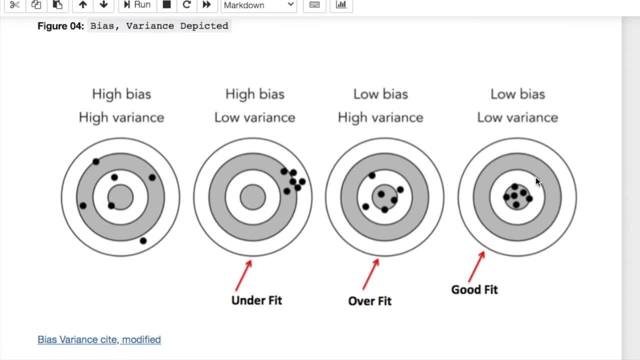 inconsistent. So the variance and bias depicted here. we would say that this is a good fit because we have low bias and low variance And your points are basically centered here. Overfitting will have a situation like this where they're kind of scattered and you're having a high variance And 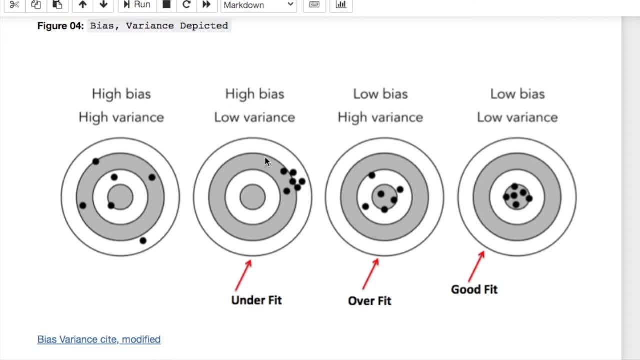 then you have the other situation, where it's an under fit. You have a variance, but you have a high bias And you'll say to yourself: well, do i always want to get rid of the variance? Well, we'll get into that, For instance when we're underfitting. if we just had 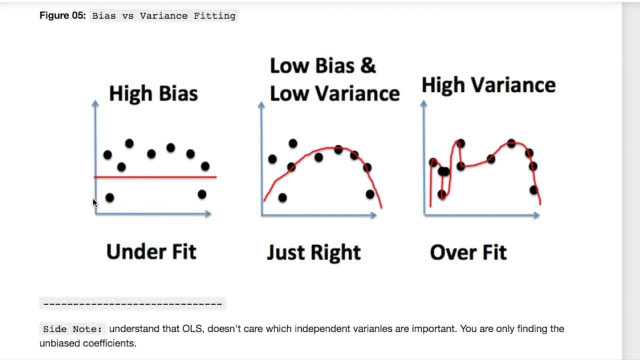 this straight line like it was linear regression, But obviously our data looked like we got this hump going on right. So obviously it's some kind of polynomial, but we didn't figure that out, So we underfit the data and now we have some high bias, Now the low bias and low variance situation is: 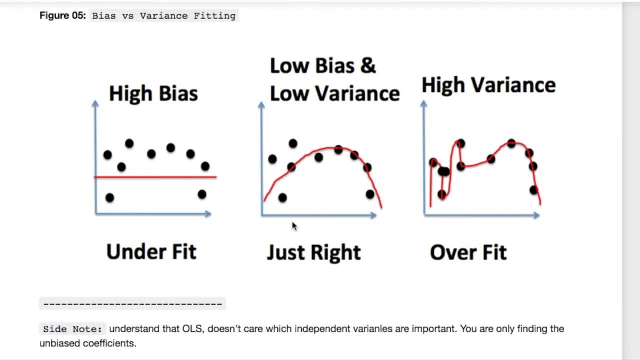 just right, And that means that we're pretty much fitting our data here and we have some outliers When we overfit and have that high variance. we're basically going about and finding every single contour of our line, approximating it to our data And we don't show any deviation with it And that's. 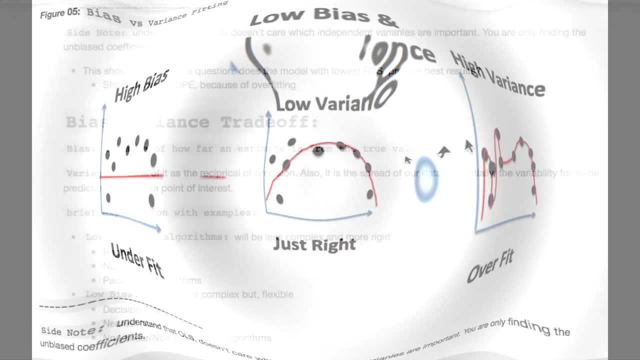 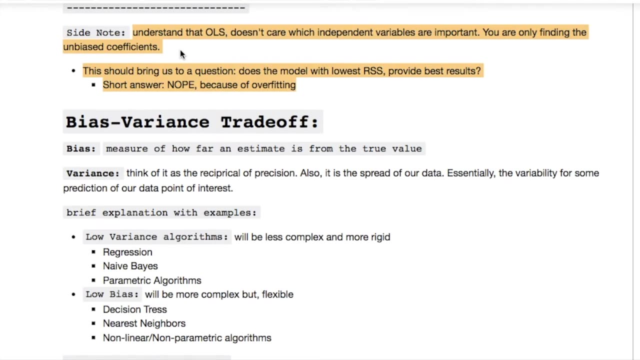 problematic, And that's something you could consider of what's going on with linear regression. A side note: understand that OLS- ordinary least squares- doesn't care which independent variables are important. You're only finding the unbiased coefficients. This should bring us to a question. 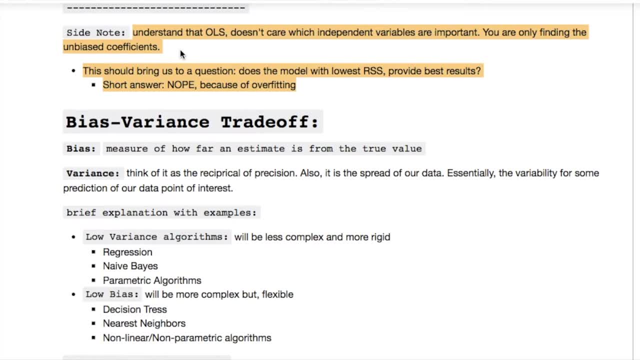 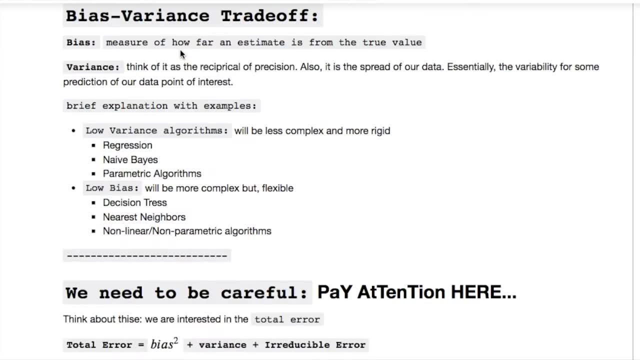 Does the model with lowest residual sum of squares provide best results? Short answer: nope, because you're overfitting. Now the bias variance trade-off is important because the bias is a measure of how far an estimate is from the true value. And you noticed above when 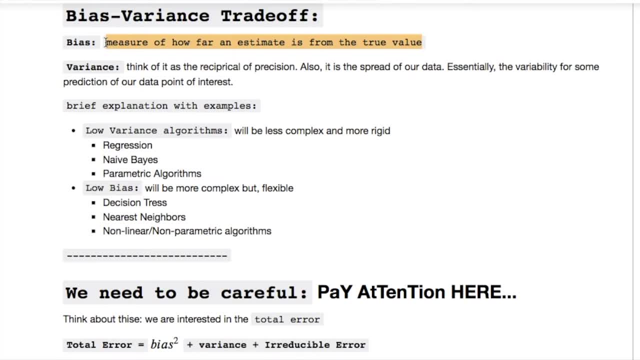 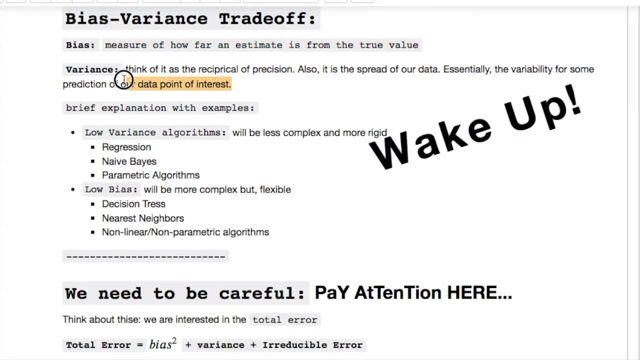 we're underfitting. our line had more error because the distance of the points were further away from the line, But it was best fit for test data. The variance: think of this as two things. One, it's the reciprocal of the precision. Also it's the spread of your data, Essentially the variability. for some. 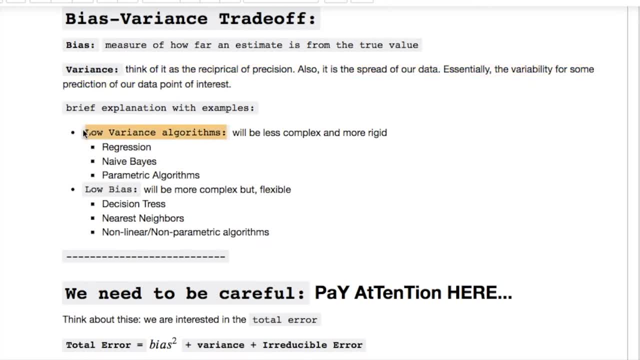 of our data points of interest. Let's look at a couple things. with low variance and low bias algorithms, For instance. low variance, we're going to have less complex and more rigid structure of an algorithm, Such as regression, naive Bayes, parametric algorithms, Whereas if we had something, 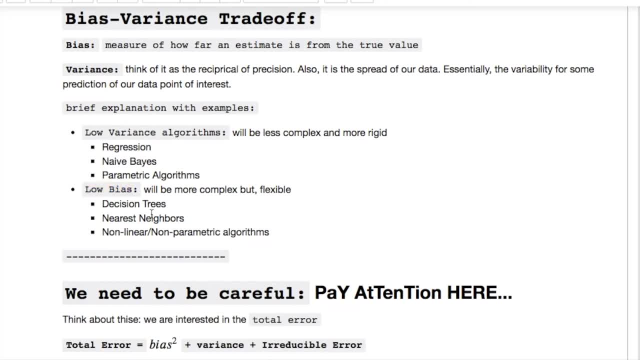 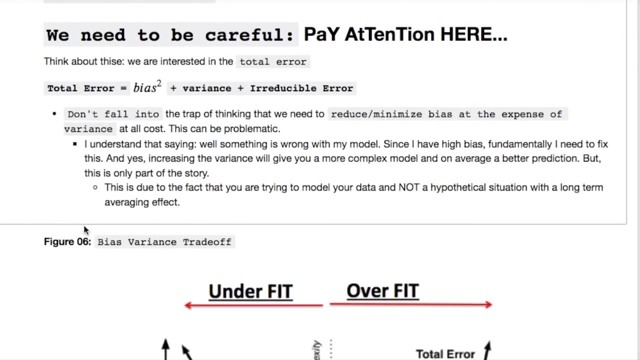 less low bias. it's more complex but it's flexible But it's flexible, Such as decision trees, nearest neighbor, non-linear, non-parametric algorithms. Please pay attention to this. We're interested in what we call the total error. Well, the total error is our bias squared plus the variance, plus some. 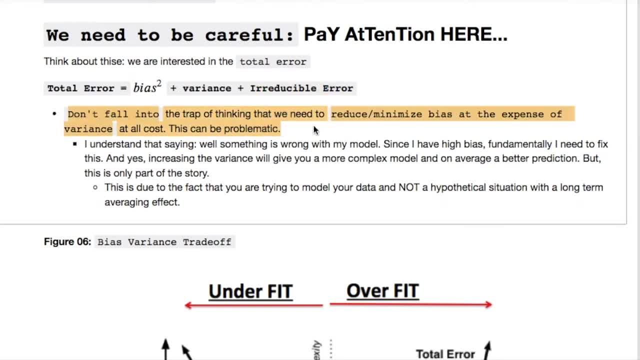 irreducible error that we can't control, And I need to highlight this. Don't fall into the trap of thinking that we need to reduce or minimize bias at the expense of variance. I need to say this again: Don't fall into the trap of thinking that we need to reduce or minimize bias at the expense. 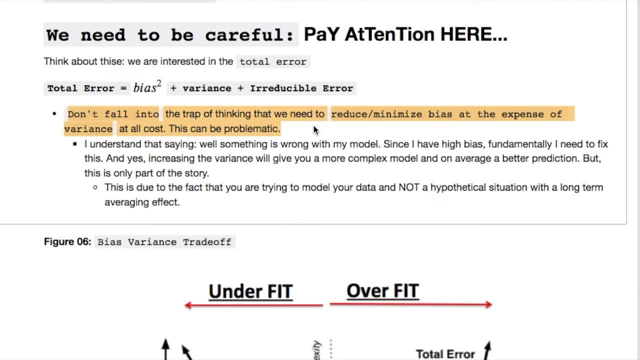 of variance at all cost. This is problematic and not good thinking. okay, Understand that I'm saying What is wrong with my model, since I have high bias. Fundamentally, I think that I need to fix my model And, yes, increasing the variance will give us a more complex model and, on average, a better prediction. 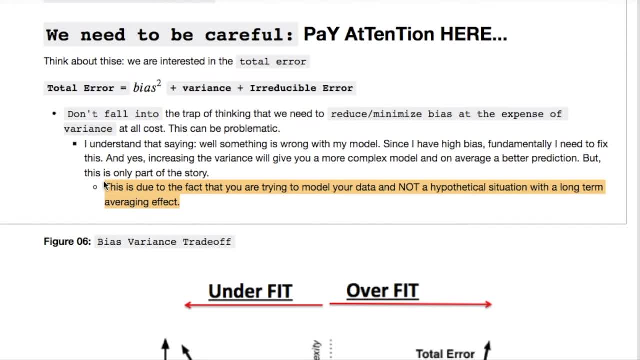 But this is only part of the story. This is due to the fact that you are trying to model your data and not a hypothetical situation with the long-term averaging effect. Hence I'm trying to model my test data. I'm not trying to get a really good model for my training data, which doesn't work on my 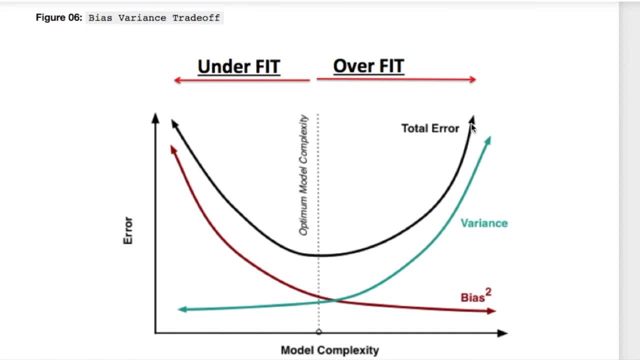 test data. Let's look at this bias variance. Here's our total error in the black line, The variance in teal blue color and the bias in the red, And this line coming down is basically in the middle. It's a little off, but that's your sweet. 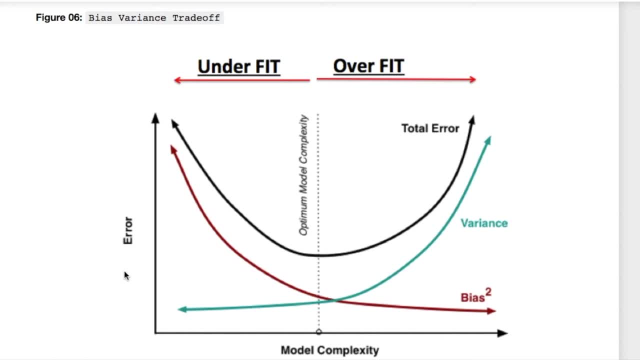 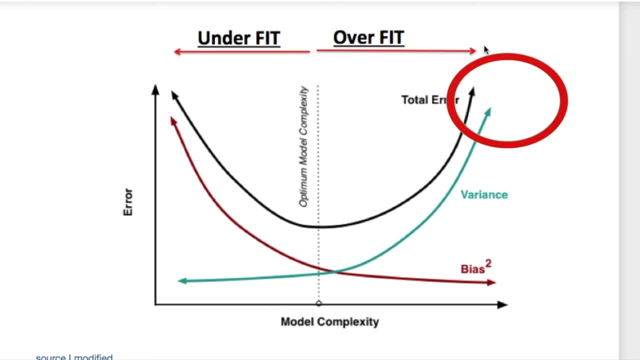 spotlight you're looking for for your model complexity. okay, We have on the y-axis your error, which is increasing, and on the x the model complexity. And when you run to the right over here, when you overfit, think of that as your ols for your linear regression stuff And going left. 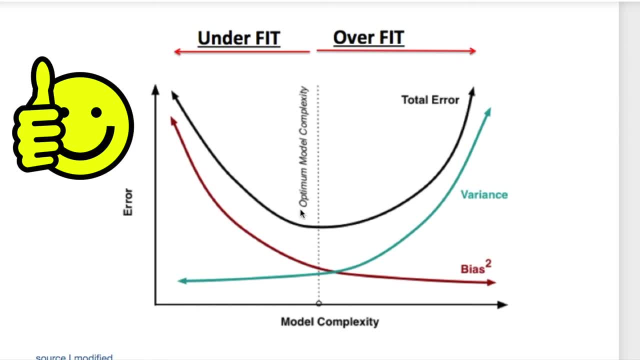 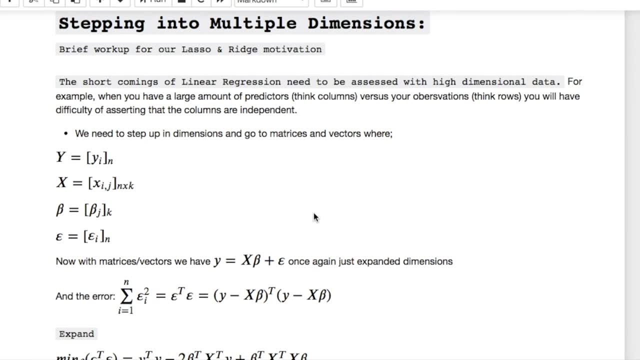 you're underfitting, which is what we're trying to kind of do. You're trying to get that half happy medium. okay, Let's look at something that we need to consider, which is stepping into multiple dimensions, Because this is where linear regression can give you some of the problems. So here's some. 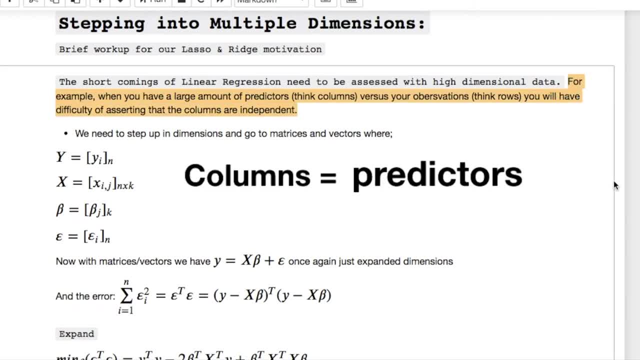 of the shortcomings with it. Let me highlight this for you. For example, when you have a large amount of predictors- Think your columns versus your observations, which are your rows- You're going to have some difficulty of establishing that your columns are actually independent. If we're setting 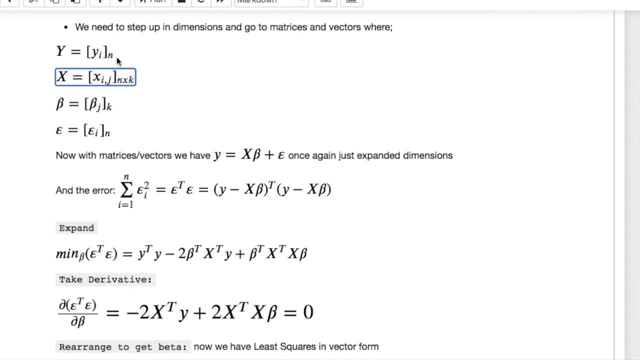 this up in our vectors. You're going to have your y, which is a n vector. You're going to have a matrix of a n by k for your x, k for your betas and an n for your errors. And if we expand our errors here, you're going to notice something We want to minimize. 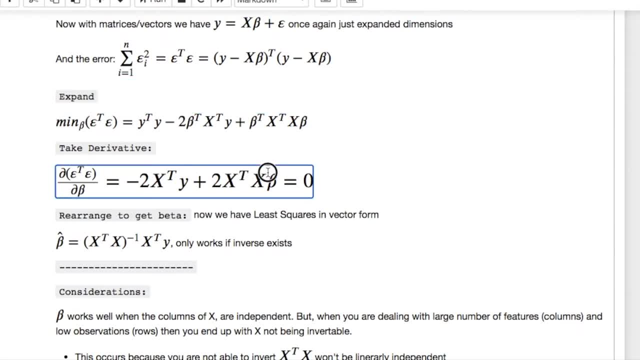 the amount of error, right? So let's expand this, Set the derivative and rearrange, And here's what our estimated beta will look like. And there's something you need to understand When you're using your matrix or your vector notation: this only works if the inverse exists. So beta works. 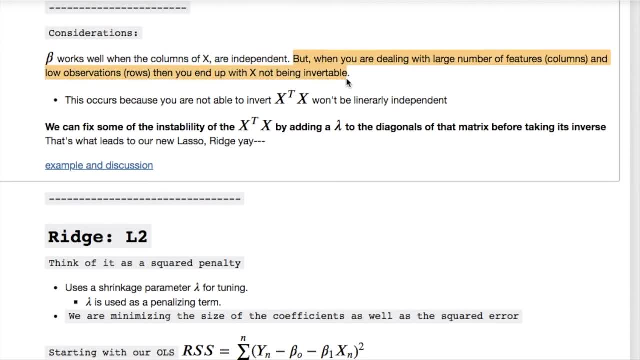 when the columns are independent, all right. But when you're dealing with large numbers of features for your columns or low and low observations, such as your rows, Then you end up having x which is invertible. So this occurs because the x transpose x won't be linearly independent. We can fix this. 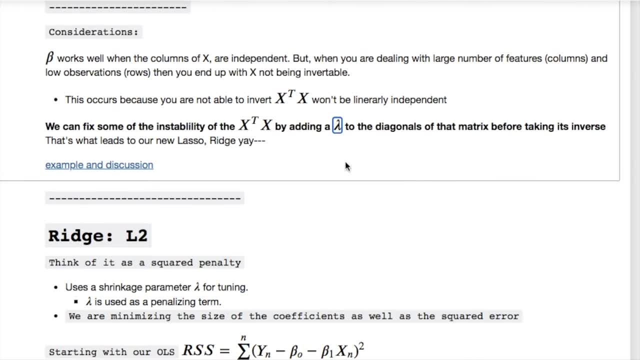 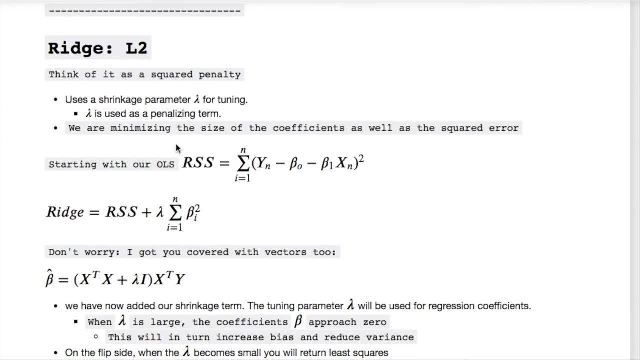 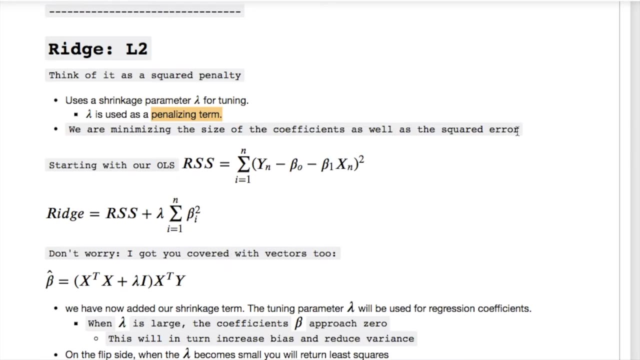 by adding a term, our diagonals, which is lambda, Which will help us. and that's what brings in lasso and ridge. Remember ridge is your l2 norm or error that you'll see. It's just a squared penalty term. It's used for shrinking. We're trying to minimize the coefficients for our standard error. 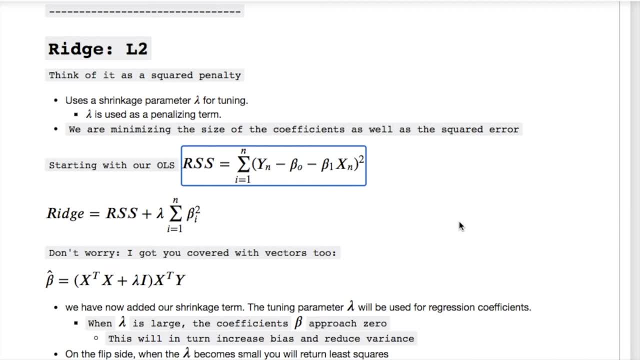 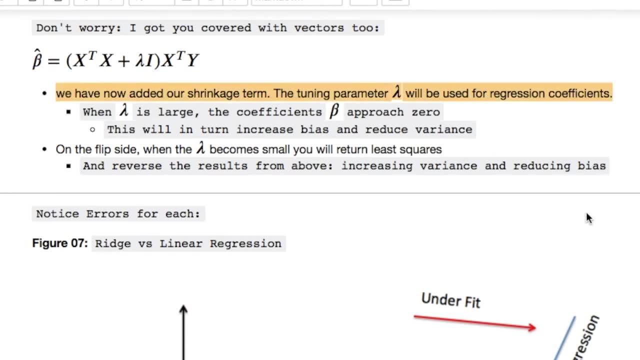 We take the same thing we had above, which is, in turn, our residual sum of squares, And we add that term on. Don't worry, I got you covered if you want your vector stuff. But just look at this. We now added our shrinkage term to the tuning parameter okay, Which is used for our regression coefficients. 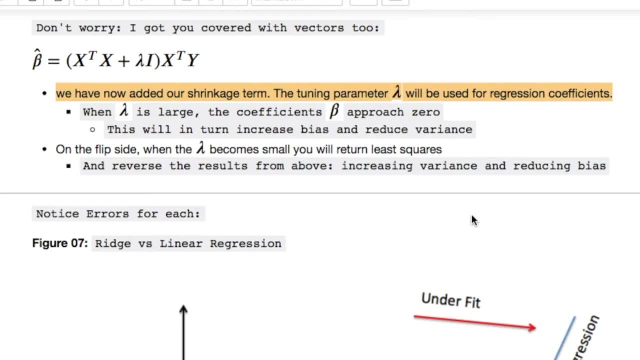 When lambda is large, the coefficients of beta approach zero. This will in turn create bias, So we're increasing your bias. When you increase your lambda, the coefficients of beta will approach zero. They do not become exactly zero with ridge. Remember that. Now, on the flip side, when lambda 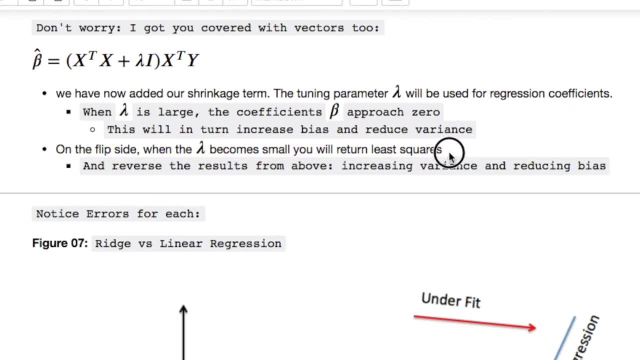 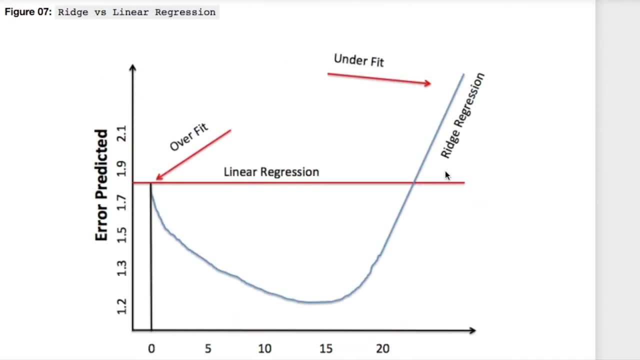 becomes quite, quite small, you approach the least squares And in this case you're increasing the variance again and reducing your bias. Here's our ridge regression. Here's our linear regression: At this point, when your lambda- let's scroll up, when your lambda is approaching infinity, you're 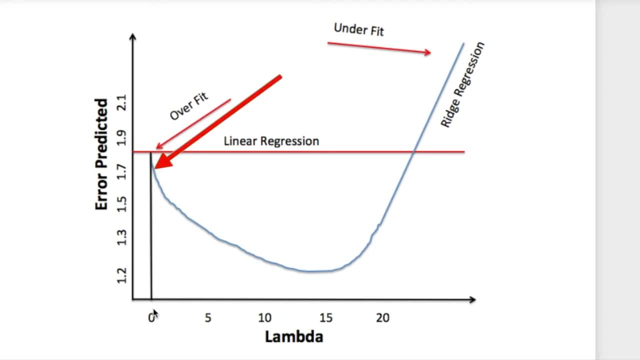 underfitting, Overfitting here, Right here where we're at zero, And we notice that linear regression has about, for this particular example, a predicted of 1.8 for our error, Whereas we have down here about a 1.2 for the ridge regression. So it means that we're trying to reduce the amount. 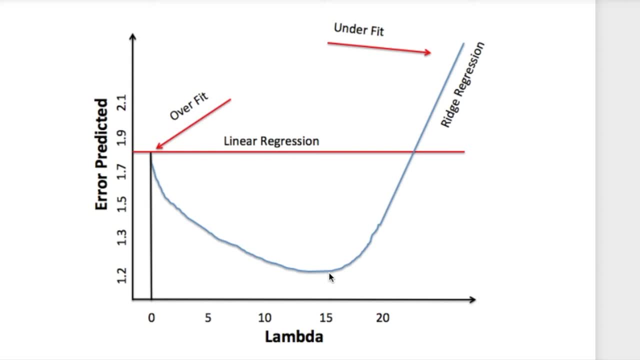 of error that we have, And in doing so, we have to use our penalty term and increase that value. So we're penalizing our coefficients in order to get this lower error. prediction Ridge reduces the complexity, not the features. Okay, you're not removing any features with ridge. Also, it's just 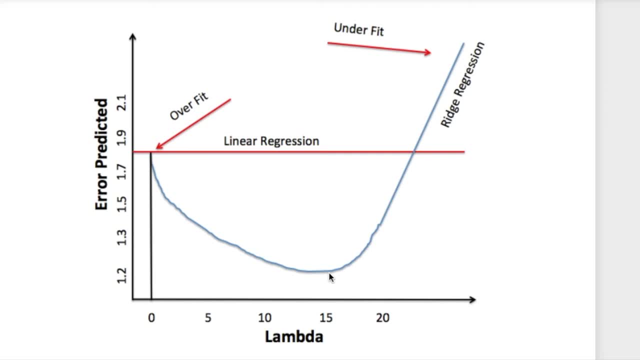 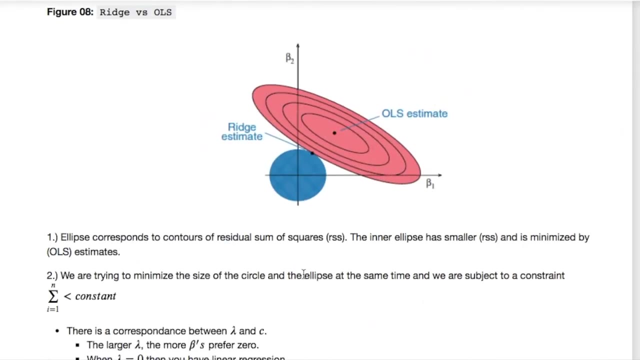 shrinking their effects And think of trying to find a new line that doesn't fit so great to your training data in order to create a better prediction overall. You may not have thought about this, but your degrees of freedom are effectively your shrinkage. It's kind of confusing, but this 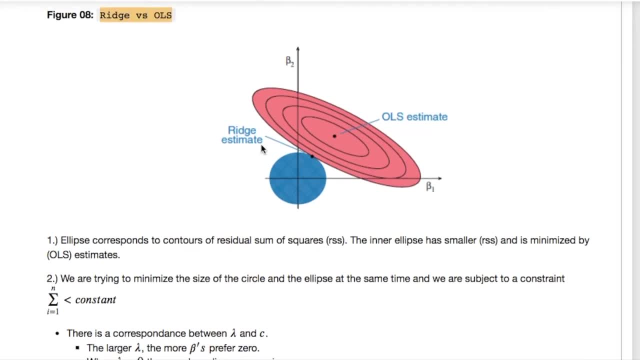 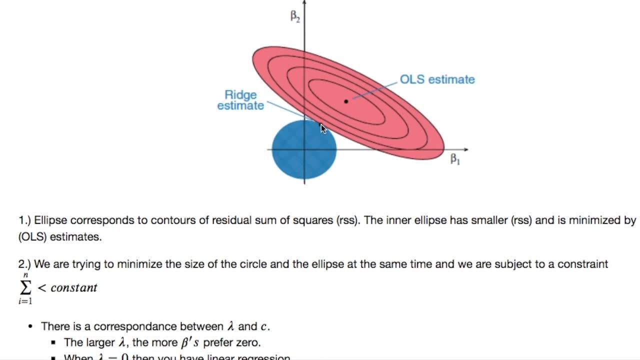 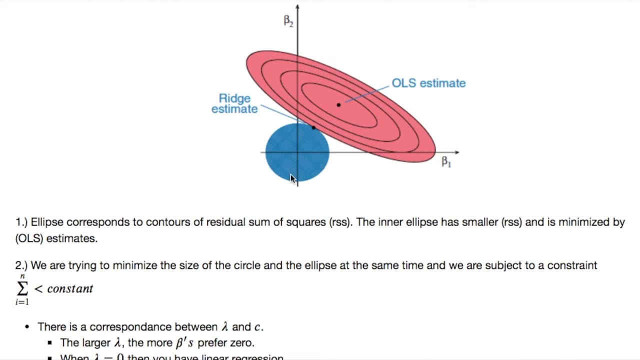 is our ridge versus our ordinary least squares. So here here, this dot, right here, this ridge estimate is what you're going to find. This ordinary least squares estimate here is our, like, optimum spot. So, basically, if you take this blue circle and increased it to that dot right here would be the optimum position, But it causes problems. 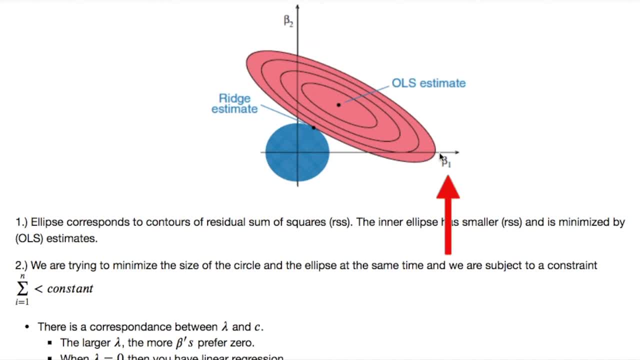 because now you're effectively changing your betas here, Because you have beta 1 and beta 2.. This ellipse contours are your residual sum of squares. The innermost one has a smallest residual sum of squares. We're trying to minimize the size of the ellipse and the circle. 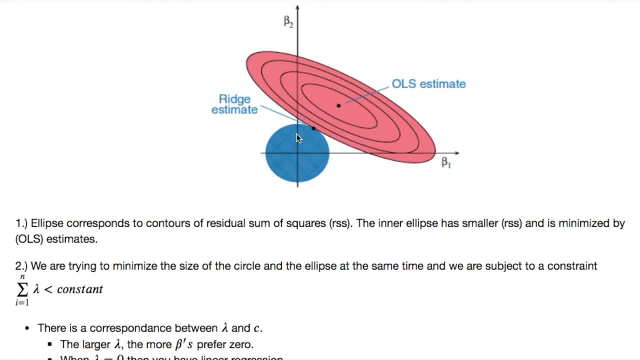 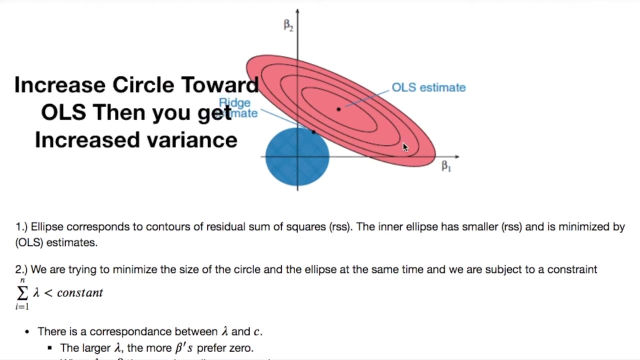 at the same time with our constraint. If you increase the size of the circle, then it's going to approach towards our best value for our OLS, But in doing so it's going to affect your betas, which are going to increase. And then now what you're doing is increasing your variance, but 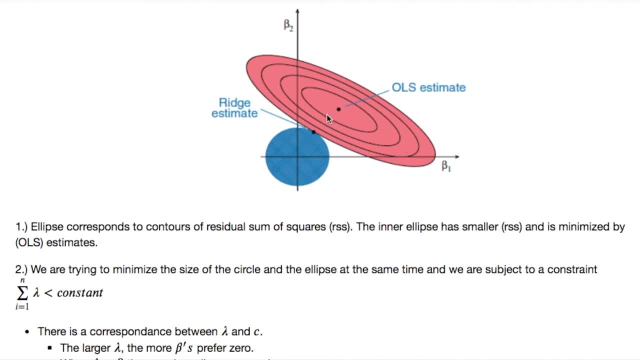 you're decreasing your error And in this case, if we make more of these contour lines And keep coming out, you would have a shrinking of this sphere, Which would mean you have more features going towards zero and increasing the amount of error. And let's think about 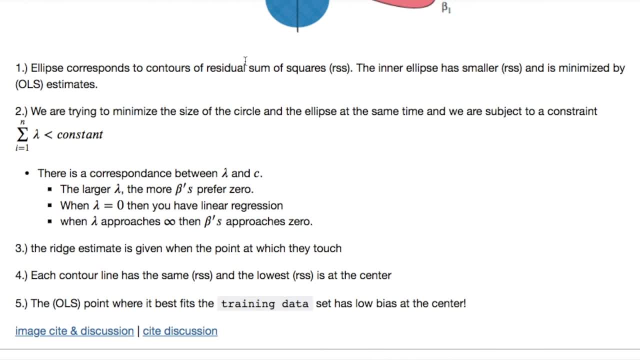 something. Let's scroll down the circle and the ellipse are constrained. So since you're trying to make both of these, minimize both of these at the same time, You have to consider something: as you increase your lambda, your betas prefer to go towards zero When your lambda goes. 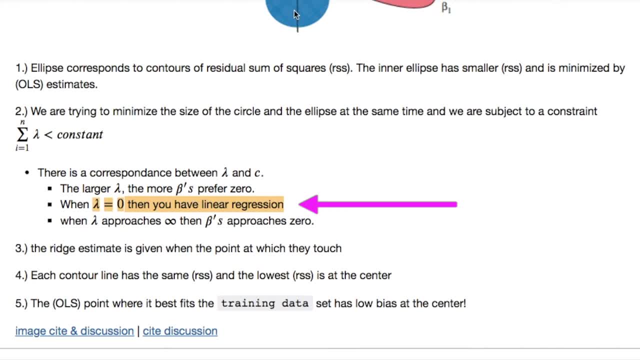 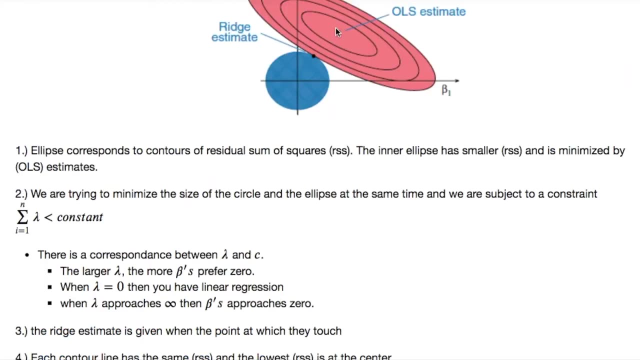 to zero, you end up with your least squares, Which means that this circle basically just shrunk into itself As lambda approaches infinity, then your betas approach zero And the ridge estimate is basically, when they touch The OLS point, where it's best fits the training, that it sets the lowest bias. 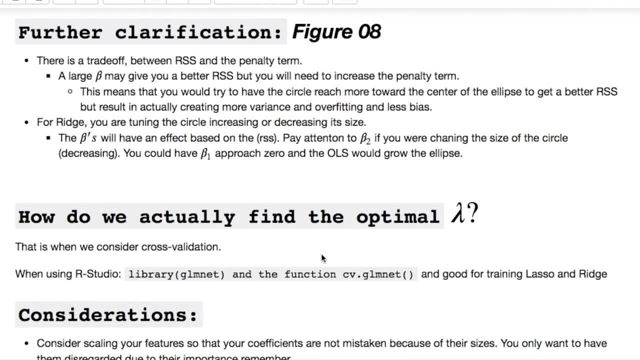 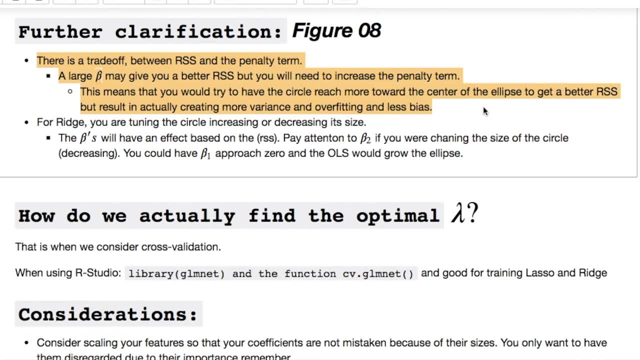 at the center here. All right, let's clarify that. that figure above Which is kind of confusing. There's a trade-off between this penalty term and your residual sum of squares. A large beta may give you better residual sum of squares, But if you're trying to minimize the size of the ellipse, 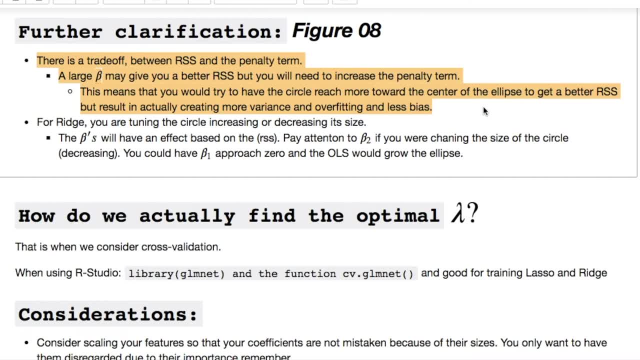 so increasing the circle, But it's going to increase your penalty term as well In order to decrease that error. This means that you would have to try to have the circle reach the center of the ellipse to get a better residual sum of squares, But you're going to end up overfitting. 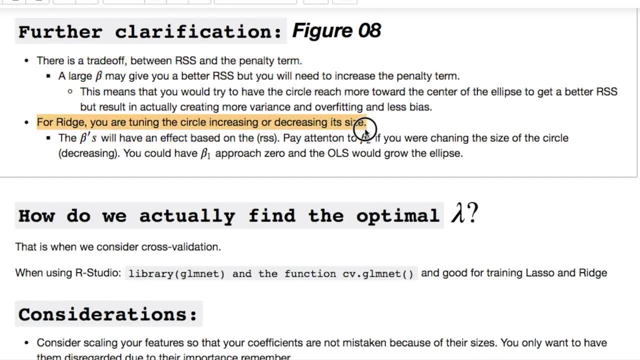 For ridge. you're tuning the circle by either increasing or decreasing its size. The betas have an effect on your residual sum of squares. Let's think about something: If we are changing the size of the circle, For instance, we are decreasing the circle and increasing the size. 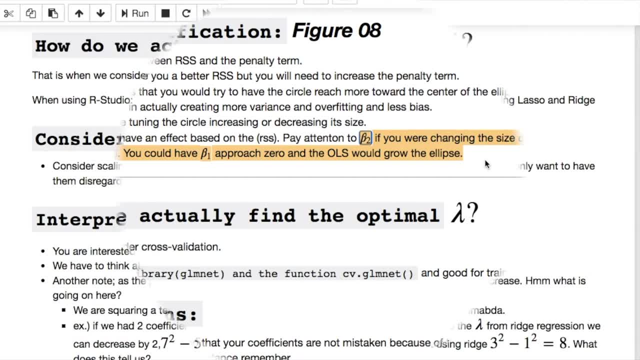 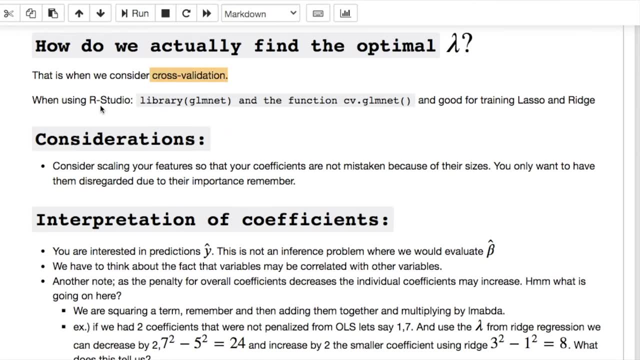 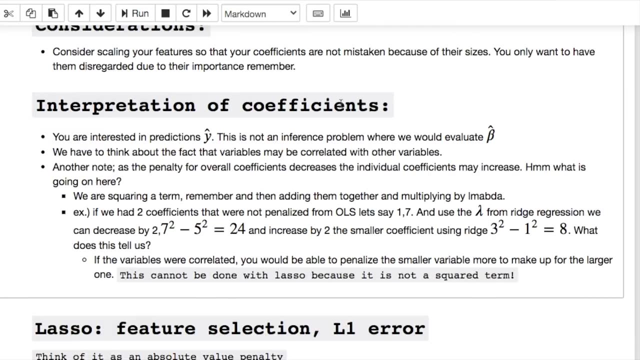 of the ellipse, Then your beta one will approach zero. So how do we actually find the optimal lambda? Well, that's interesting because you consider cross-validation In the case of Rstudio. use glmnet for your library and then call the cross-validation function from there. Here's some. 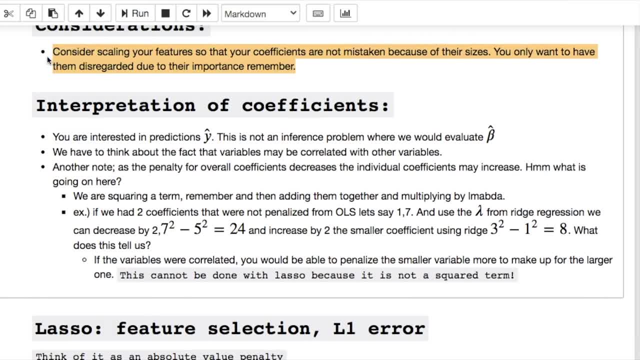 considerations. I said this before and I'm saying it again: Consider scaling your features and centering So that your coefficients are not mistaken because of their sizes. You will only be able to do this if your coefficients are not mistaken due to their importance. Remember not. 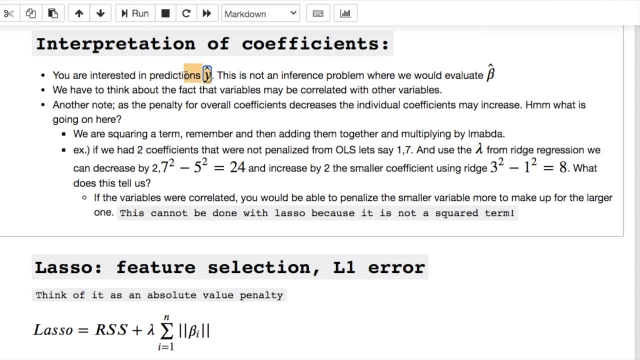 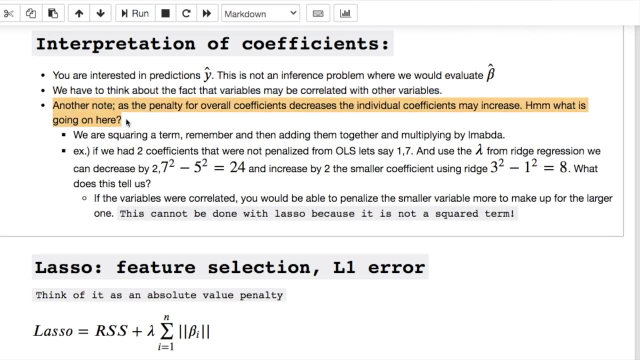 due to their magnitude. Interpretation of your coefficients. You're interested in predictions of your y. This is not an inference problem. where you're looking to evaluate your beta hat, We need to think about the fact that the variables may be correlated. Another note as the penalty for 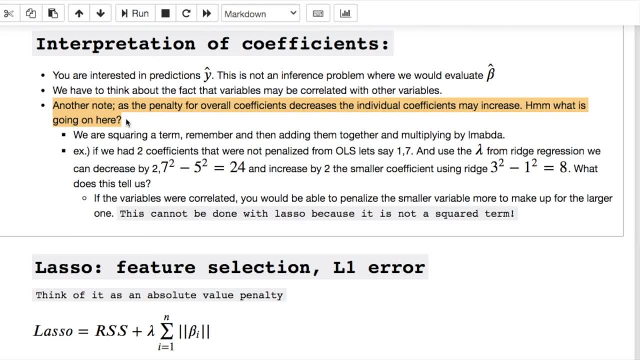 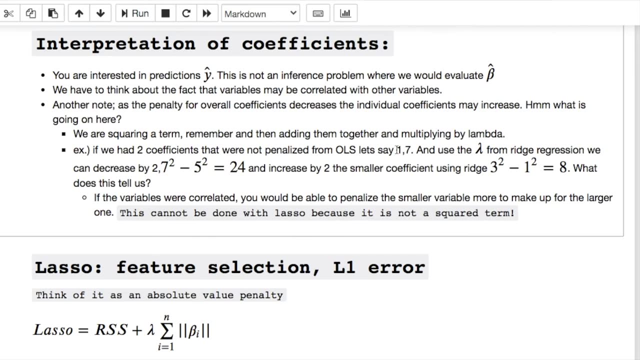 overall coefficients decreases, the individual coefficients may increase Again. overall coefficients may decrease, The individual coefficients may increase. But what is going on with that? You're squaring your terms, remember, And you're adding them together. If we had two coefficients that were not penalized from. 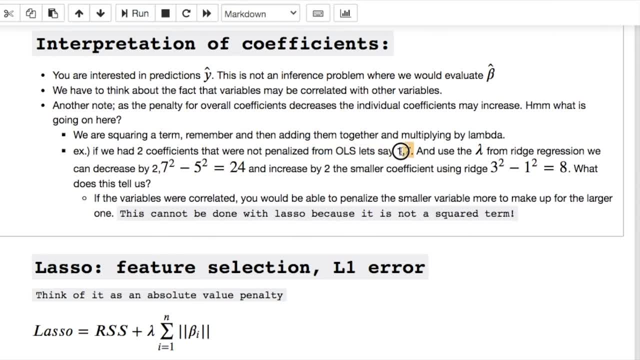 the original least squares Say, we had one that was seven and one that was one. And we use our lambda from ridge regression. Let's say we're decreasing by two, We end up with 24 here and the other one, we'd end up with eight. But what does that tell us? If the variables were correlated, you'd be able to. 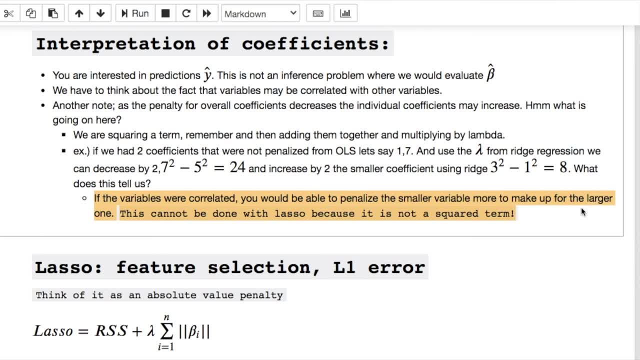 penalize the smaller variables. If the variables were correlated, you'd be able to penalize the smaller variables. If the variables were correlated, you'd be able to penalize the smaller variables. So we're going to use the last variable more to make up for the larger one. This cannot be done with. 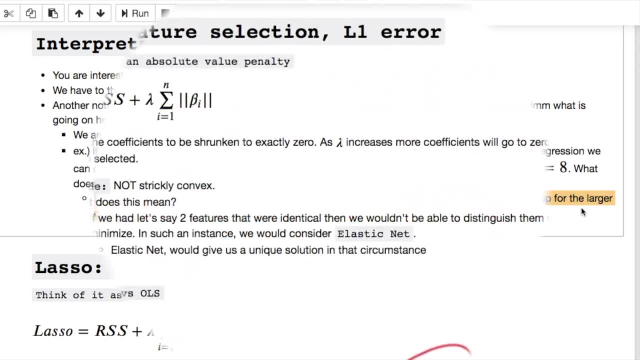 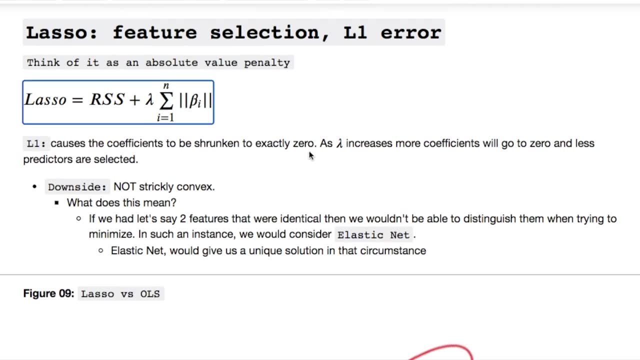 lasso, on the other hand, Because you do not have squared terms. Lasso, on the other hand, is going to be your l1 norm or error. It's just the absolute value of it right here, And this causes the coefficients to exactly shrink to zero. As you increase lambda, more coefficients will go towards. 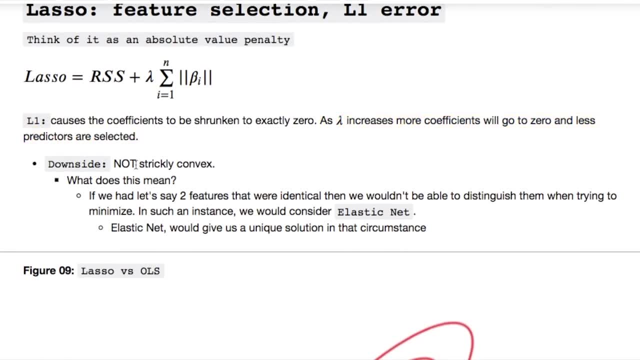 zero and less predictors are selected. The downside of this is not strictly convex, And what does that even mean? If you had two features which were ideal, If you had two variables which were not features which were identical, then you want to be able to distinguish them, to do a minimizing. 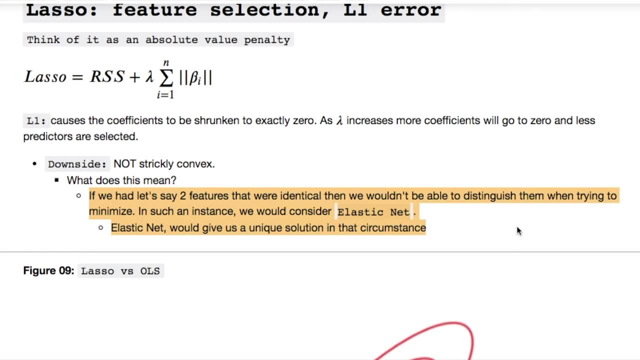 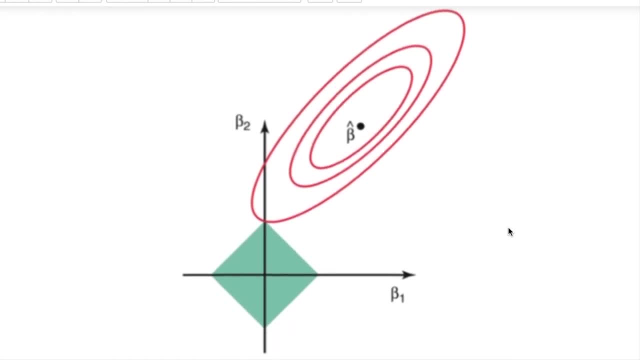 And in that instance, you would need to use elastic net, which would give you a unique solution in that circumstance. So let's look at ols, verse our lasso and you notice it's not a circle, it's a diamond shape. now There's a slight difference with this diamond shape. okay, since we're doing feature, 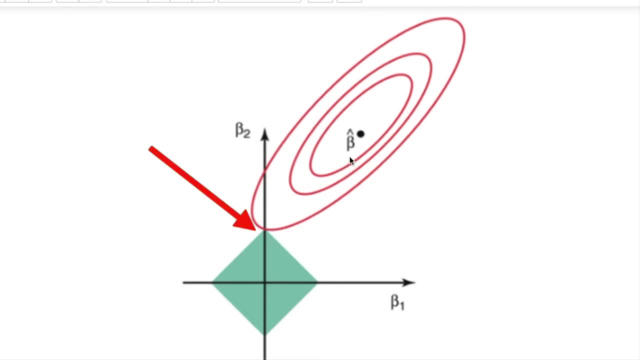 selection, The tip of the diamond when it reaches that ellipse- that's the coefficient corresponding to the axis- that will be shrunk to zero Notice. this is a 2d situation. if we had this increasing in dimensions, you would have more of these diamonds protruding outwards in different 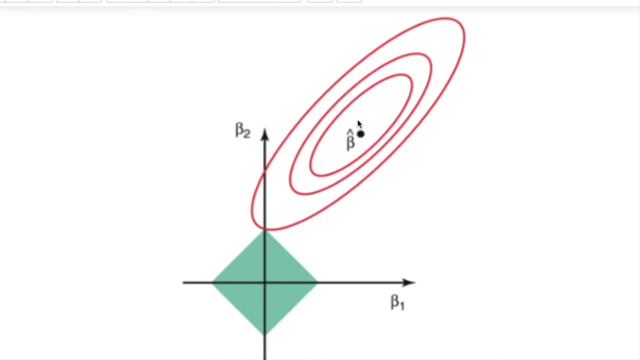 dimensions, which would give us the ability for the corners to approximately touch more often to that ellipse, which would potentially shrink more coefficients to zero. If we created more of these rings, made this diamond smaller, we would lower our betas and have more of these diamonds protruding outwards in different dimensions. So this is a 2d situation. 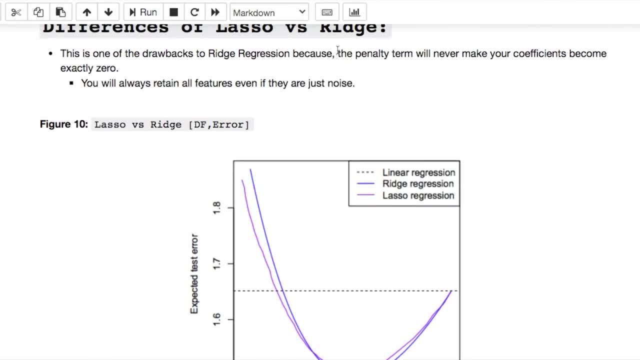 where you would have more error. So let's look at this a little bit more. Here's a difference ridge: the penalty term will never make your coefficients exactly zero and you're always going to retain all of your features, even though you may have just noise. This dotted line, horizontal, is our linear. 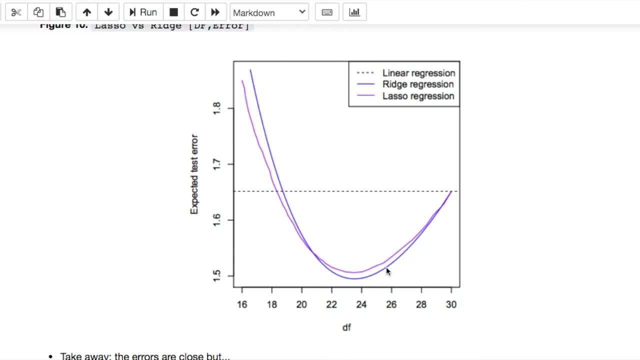 regression. the purple one is our lasso and the bluish purple one blue one is your ridge. Here's the takeaway from this: we're using our dfs on our x-axis and our expected error. Think of your df as your shrink And on average, you have around 24 features selected using lasso, whereas ridge you have. 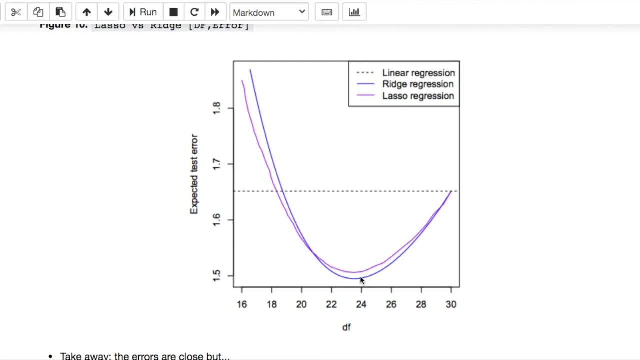 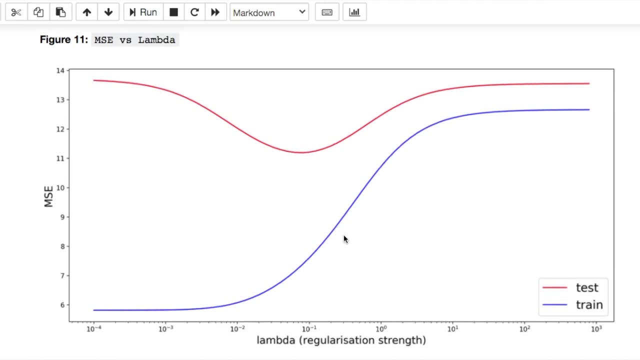 all of the features at all times used. That's something to take note of. Here is an example using ridge, where we have your mean squared error versus your lambdas, and there's a few things that you need to notice with this. The first thing, here's our test data- this little. 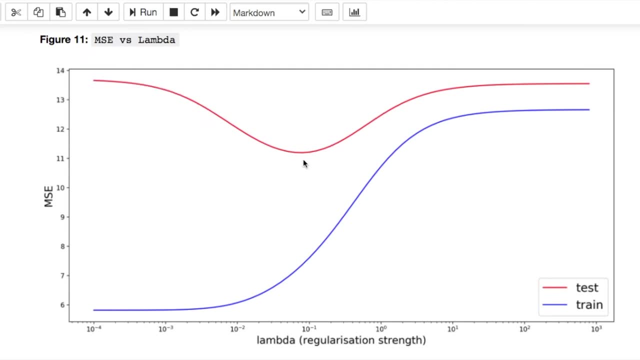 hump right here where it's convex. this is our optimum point that we want. We're going to know that this training data starts at the bottom here, which is really low error. We have a higher error here at the start for test data, suggesting that we have overfitting At this point right here. this: 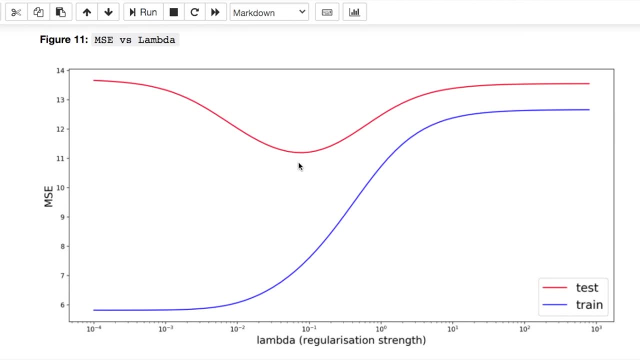 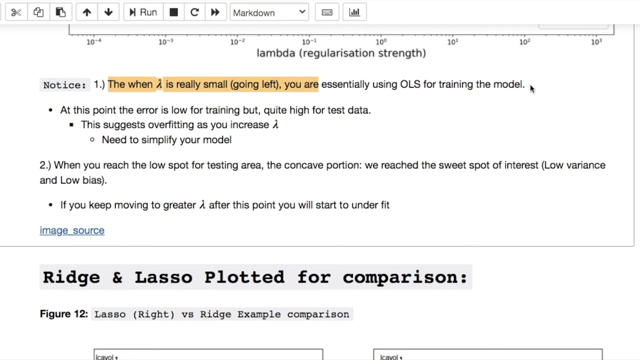 suggests where we have the best variance and bias trade-off: Our low variance, low bias. After this point we start to have issues with under fitment. So that's the takeaway, This recap: when you have a really small value for lambda, essentially you're going towards the linear regression. So that's the 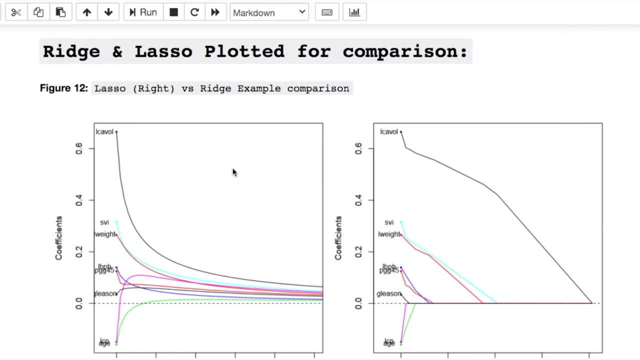 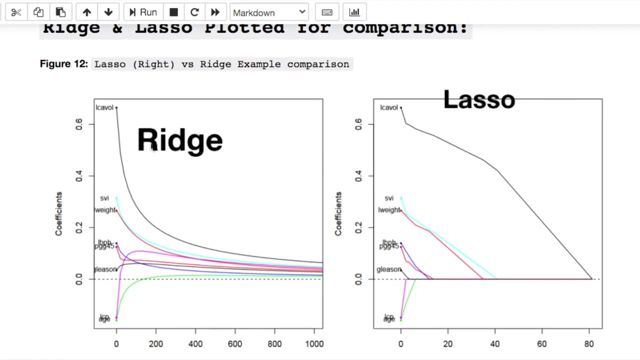 linear regression. Let's look at the comparison of ridge and lasso, plotted in respect to the coefficients, versus the lambdas. On the right side, this is your lasso. On the left side, this is your ridge. Ridge will approach zero. Never set your features to zero. You noticed here that these three 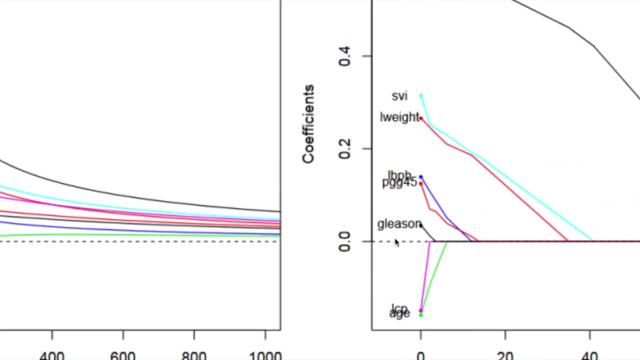 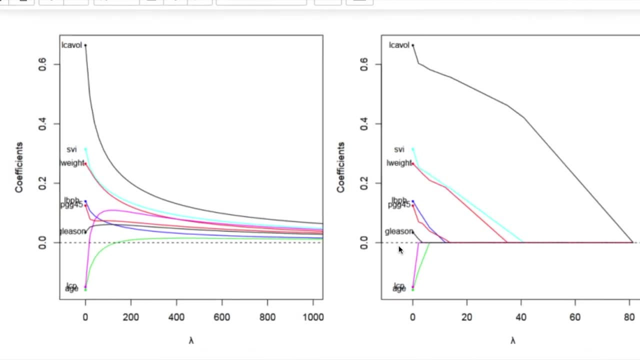 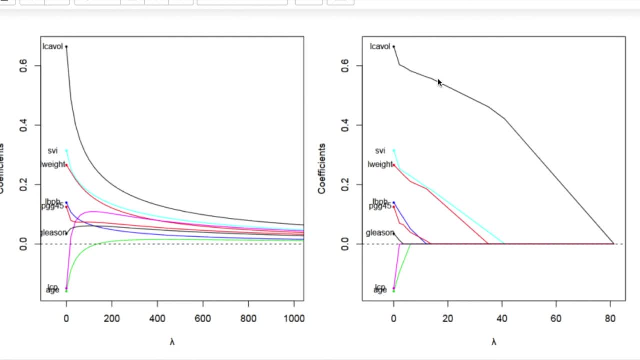 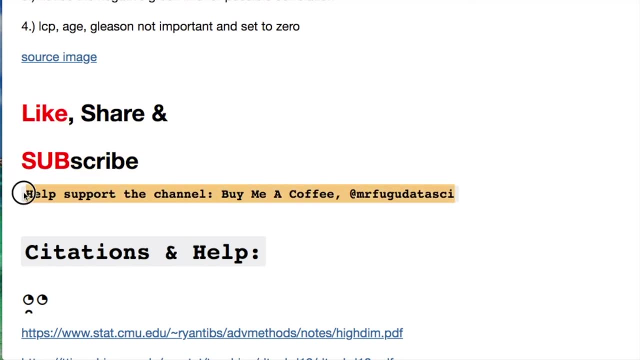 say which of these features are important to remember. cross validation would be the use case of that, But, as always, I'd like to say: please like, share and subscribe, and if you subscribe, turn on that notification bell If you thought this is useful and would like to support the.